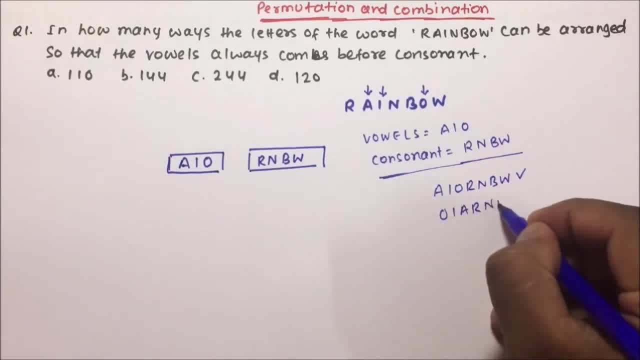 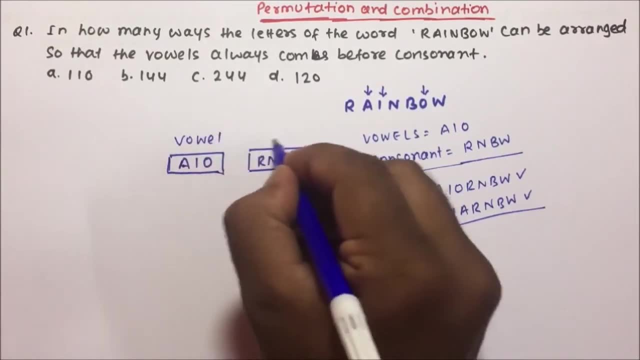 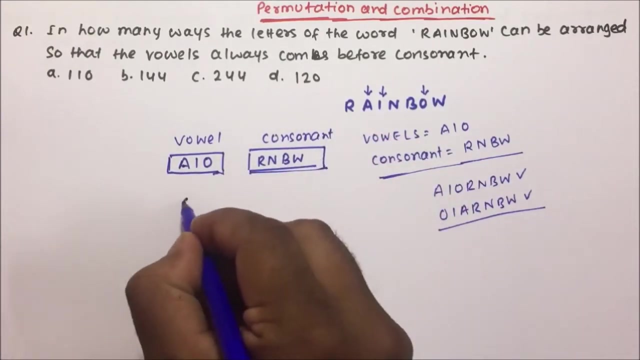 we can have a word: o, i, a, r, n, b, w, so this also, so like this words we can have. the only condition is it should start with vowel. vowel should come first and then consonant should come later. consonant should come later. right, friends? okay, so there is only one way. so, there is only one way. it. 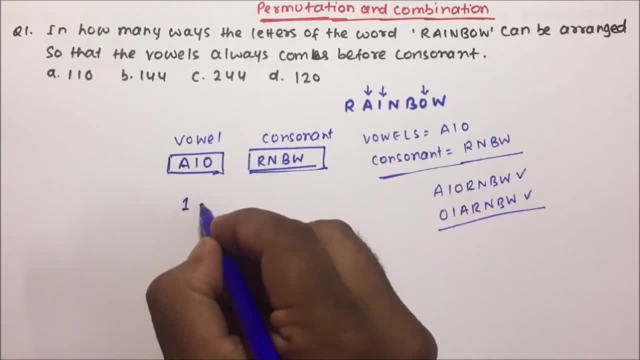 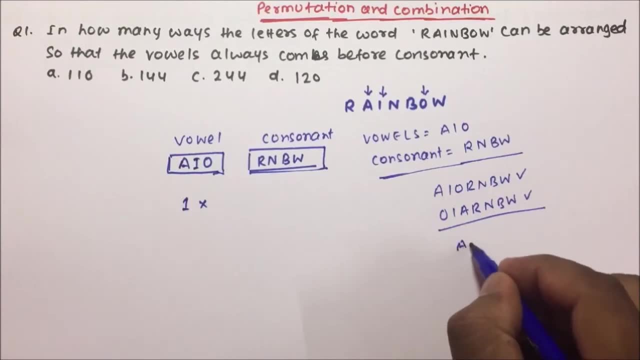 can be arranged. i mean vowel will come this side and consonant will come this side. but friends, these vowels, these vowels will get arranged among themselves. what i want to say is see, friends, the word can start with a, the word can can start with i, the word can start with you know o, so among them. 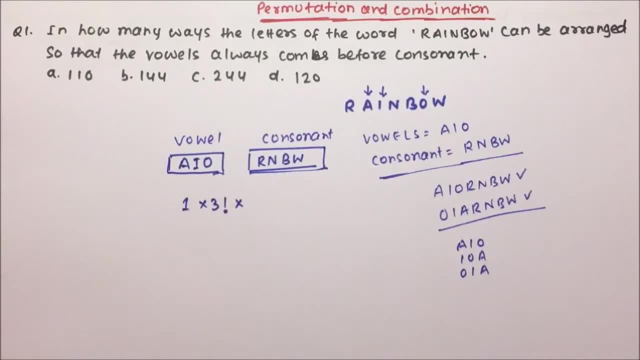 they will get arranged. see three different words. so three factorial right. three different word means three factorial, so among them they will get arranged in the three factorial ways. if you want, i can show you. so one more words. you can have a, o, i and then i a. 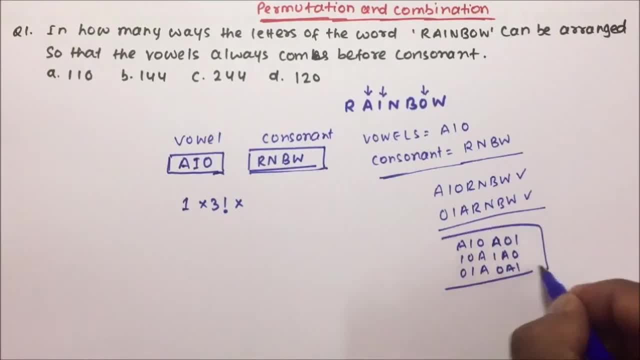 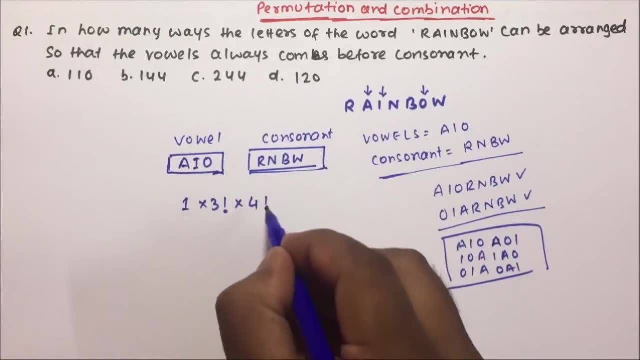 o and then o, ai. so there are the. this is a six. this is a six ways in which vowels we can write it. and now, if we talk about the consonant friend, then four different consonants, it will be four, factorial now three. factorial is three into two and four. factorial is four into three into two. 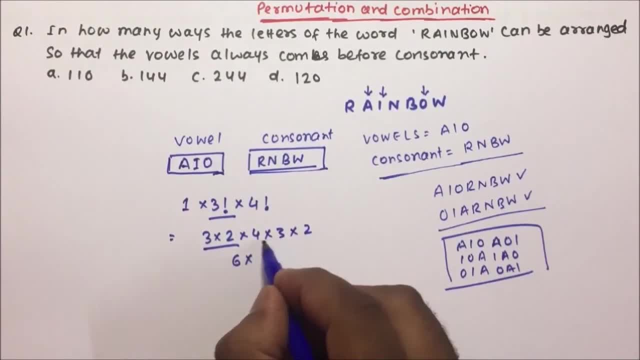 so this will be six and four into uh, three is twelve. twelve into two is twenty four. right, see four factorial. four into three is twelve and twelve into two is twenty four. that means total 144 ways. so we have total 144 ways in which, if you write the, if you write the word, 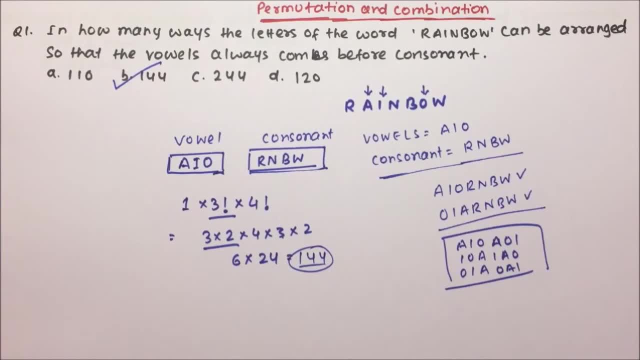 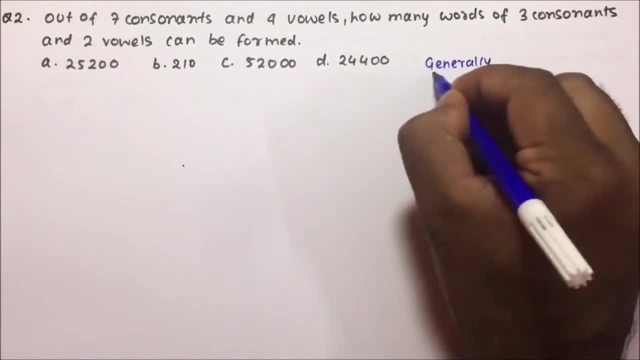 then vowels will come before the consonant. right friends, now moving towards the question number two. question number two is a very good question. generally, student will do the mistake here. so that is the only reason i am telling this question is a very good question. so let's see. 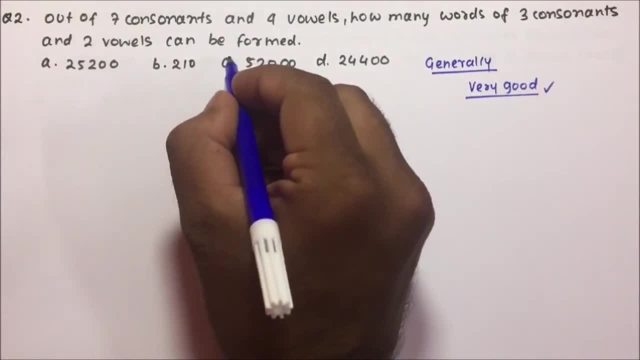 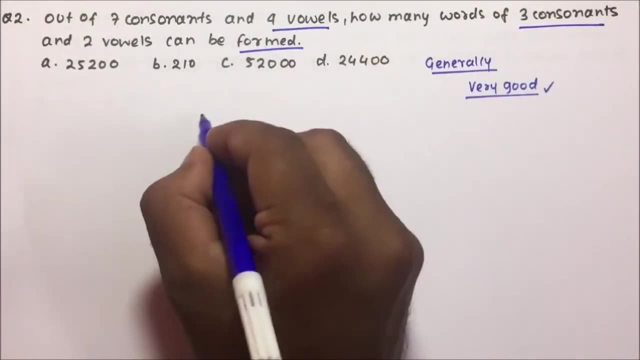 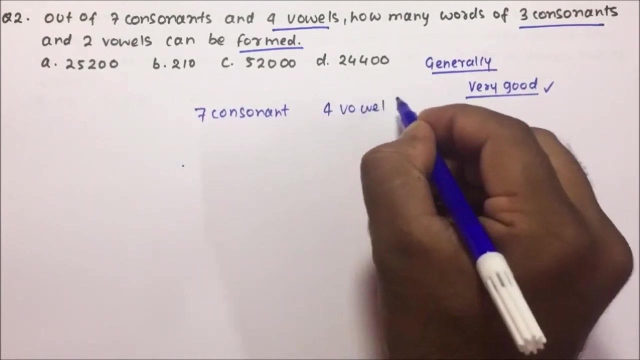 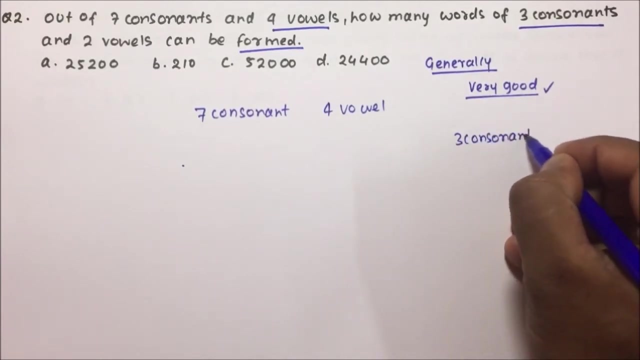 how we are going to solve this question. so, out of seven consonant and four vowels, how many words of three consonants and two vowels can be formed? so, friends, we have total seven consonant and four vowels. okay, now we have to form words using three consonant, using three consonant and two vowels. so we have to. 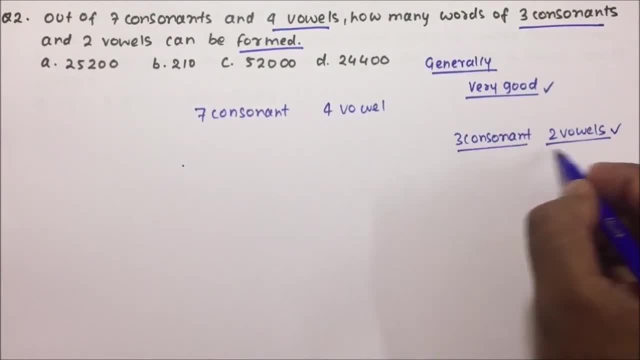 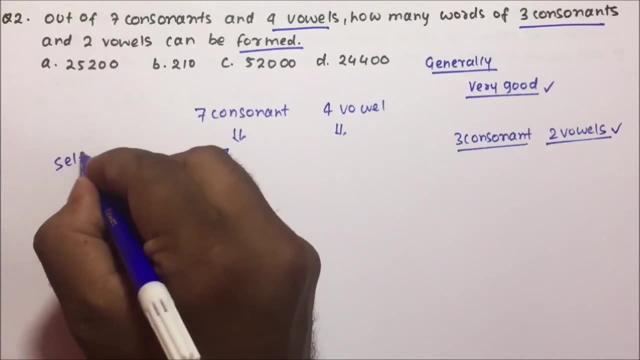 so we have two friends, so we have to form words using three consonant and two vowels. so the first thing what i am going to do is i am going to select. so the first thing what i am going to do is i am going to select. so select means nothing, but 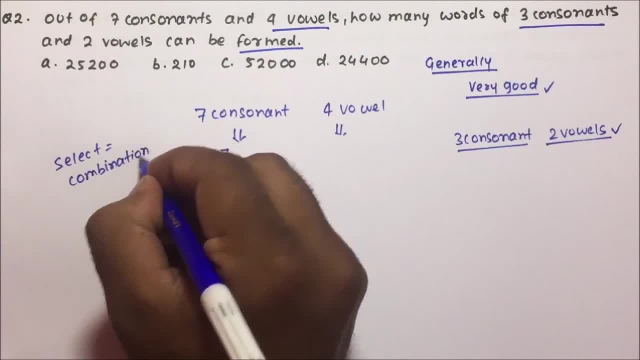 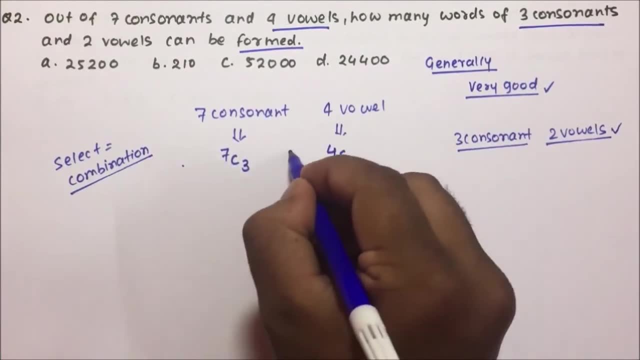 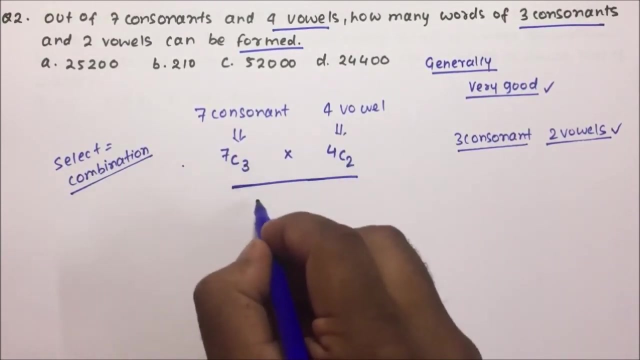 combination. so select means nothing but combination. so, friends, i am going to select three, i am going to select three consonant, and here i am going to select two consonant. so in how many ways i can select? so seven c. three into four c two, okay, so let's solve this. so seven c. 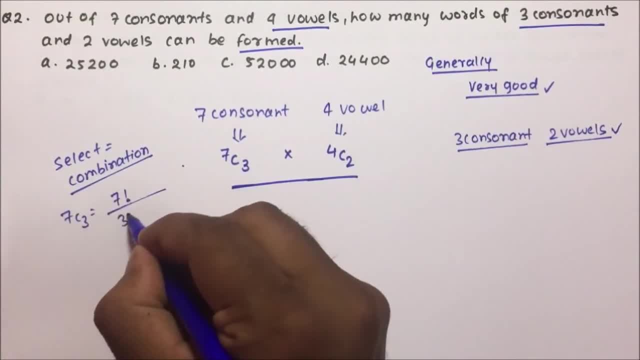 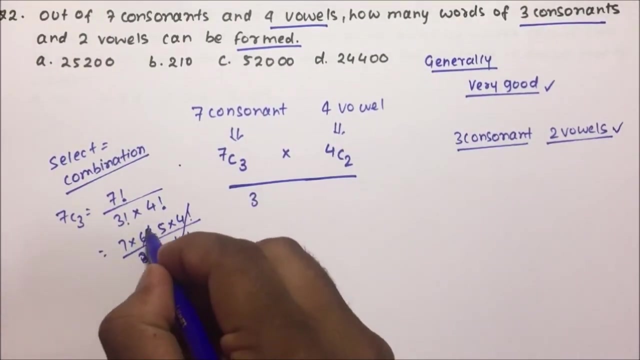 three. how can i solve seven factorial divided by three factorial? this is a formula, and seven minus 3 will be 4 factorial. so 7 into 6, into 5 and 4 factorial will write like this: and then 3 factorial will be 6 and 4 factorial will write as it is now: friends, 6 and 6 will get cancelled. 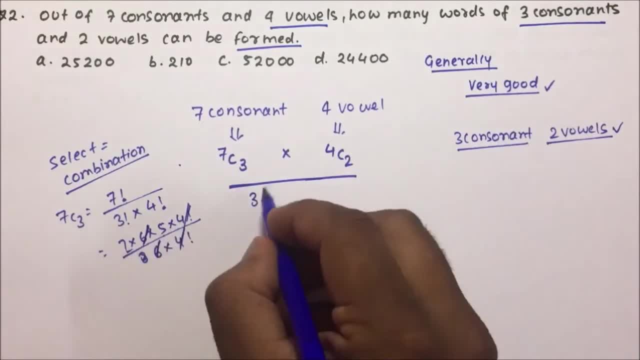 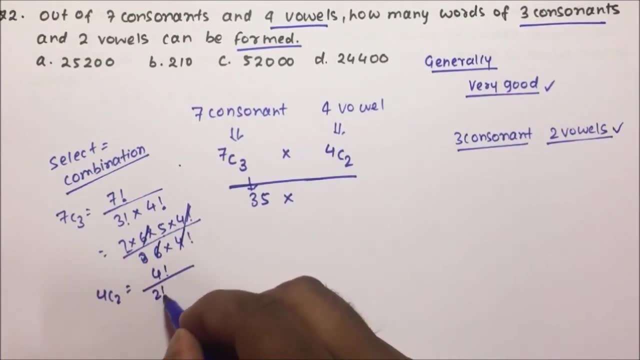 and 4 factorial and 4 factorial will get cancelled, so 7 into 5 will become 35. so this value, we got 35 and 4 c 2. so 4 c 2 means 4 factorial divided by 2 factorial into 4 minus 2 is again 2 factorial. 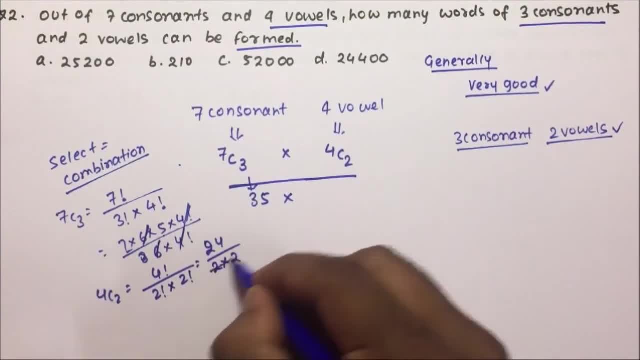 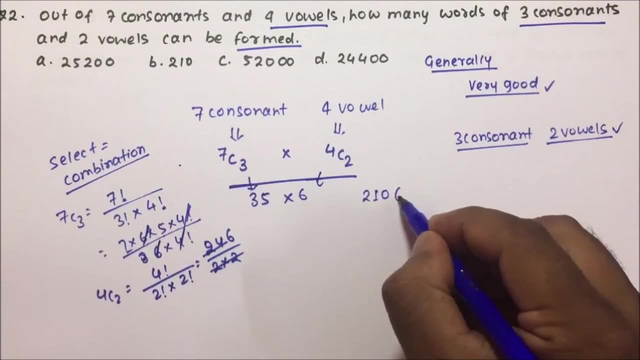 so 4 factorial is 24 divided by 2 into 2. so this will divide this by 6 times. so 35 into 6 is 210. so there are total 210 ways. so there are total 210 ways, are there friends? there are total 210. 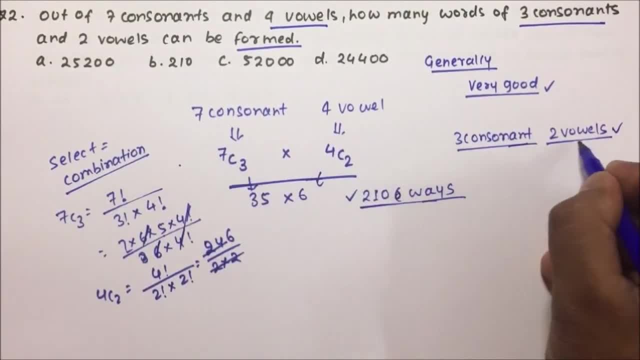 ways are there, friends, in which we can select three consonant and two vowels? so now i have three consonant and two vowels. now i have it right. okay, friend. so do not mark the unaccompanied and unaccompanied. so do not mark the unaccompanied and unaccompanied. 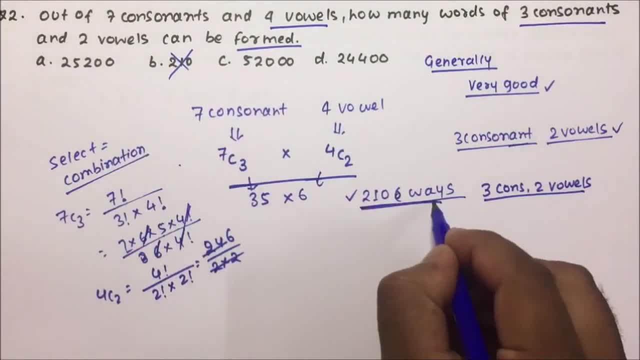 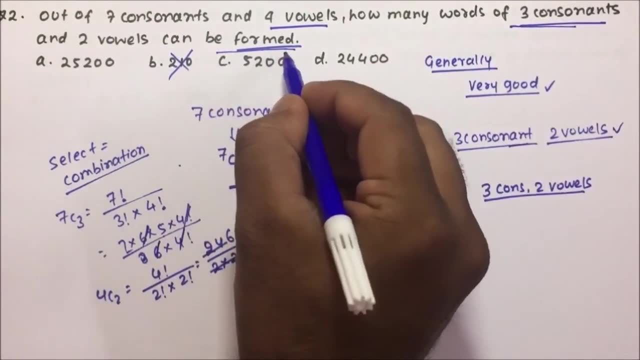 answer is 210. it will become wrong, because there are 210 ways in which we can select three consonant and two vowels. but now we have to arrange. permutation means arrangement. so now, friends, we have to arrange. so we have five different letters, so we have five different. 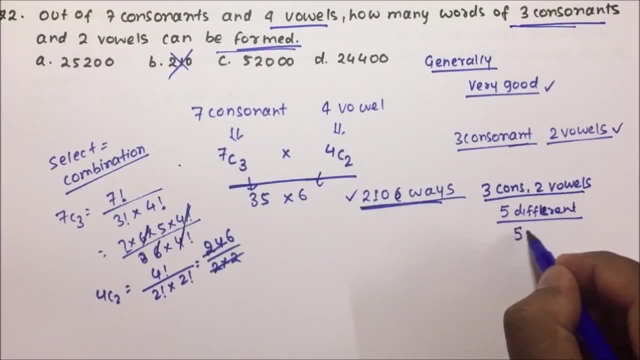 letters and the five different letters can be arranged in 5 factorial. so the total number of ways, so the total number of ways, will become 210 of ways, so the total number of ways can become 210 into 5 factorial, so 210 five factor will be. 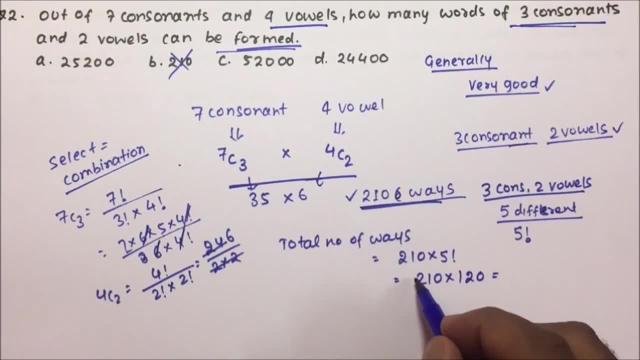 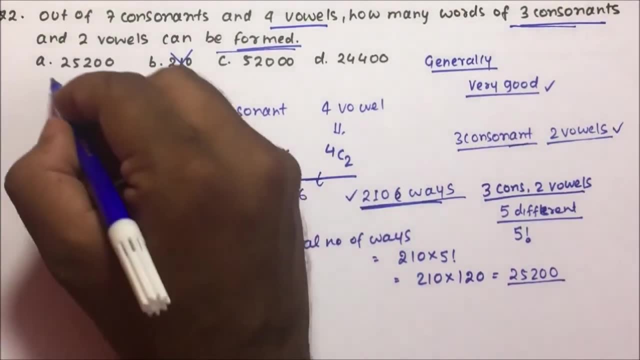 11112 into 20 will be 240, and 240 plus 12 will be 252 and with 2, 0 will come. that means 252 and then 2, 0 will be the correct answer. so this was a very good question. generally, what? 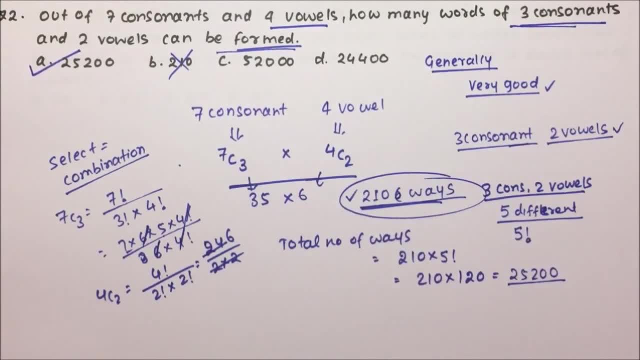 a student will do, they will just select. they will just select three consonant and two vowels, but they will not arrange it. but clearly they are asking how many words of three words give um. this is crazy, this is a difficult one. so this is a difficult answer and it is hard, right and gently um. 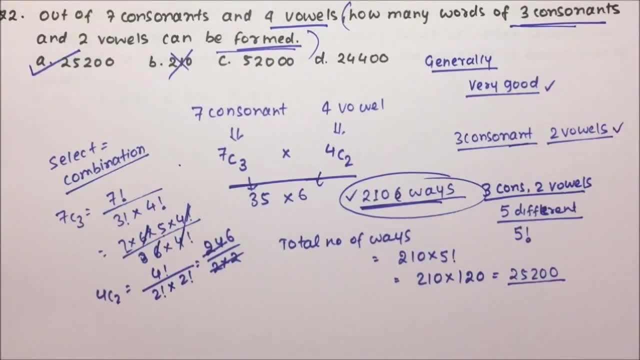 of three consonant and two vowels can be formed. So, friends, I hope you would have understood this question. this was a very important question. 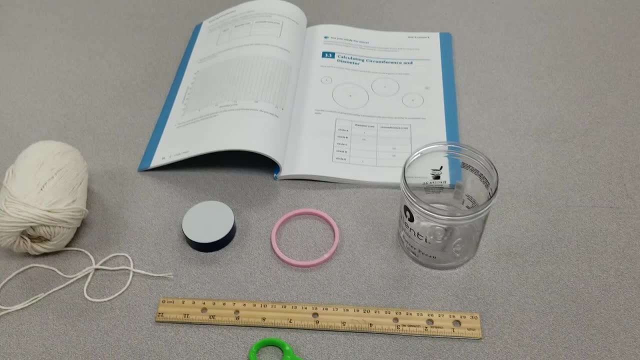 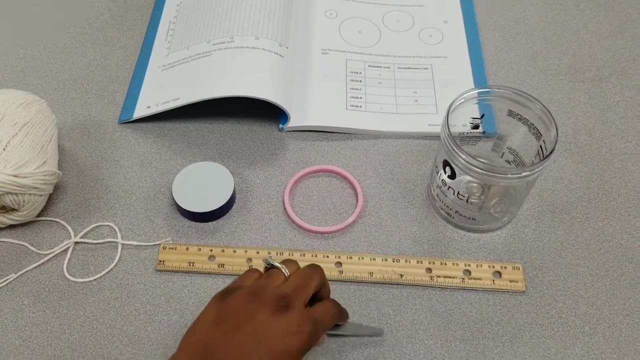 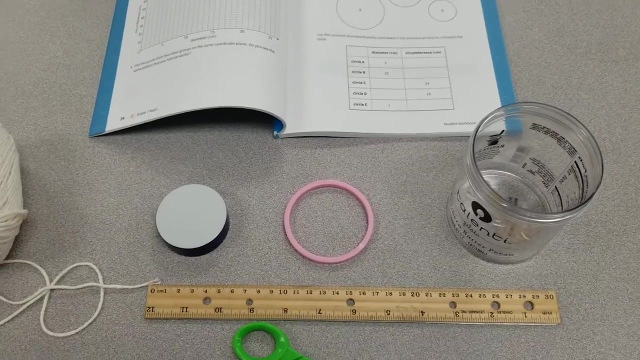 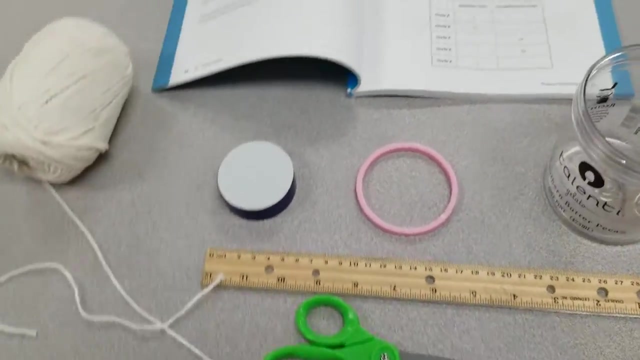 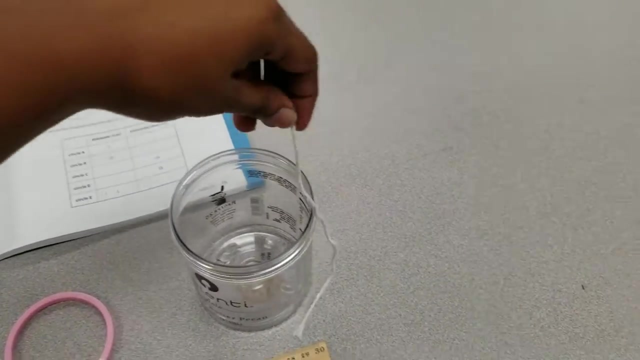 My blue textbook, a ruler and scissors. I need to get the circumference and the diameter of all three objects and record them in my book. I'll also need string for this. So the first thing I want to do is choose an object and take the string and wrap the string all. 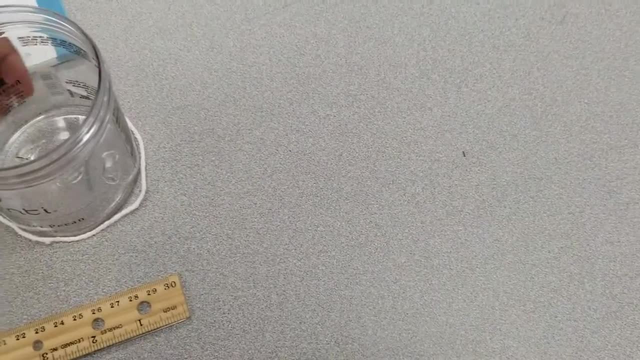 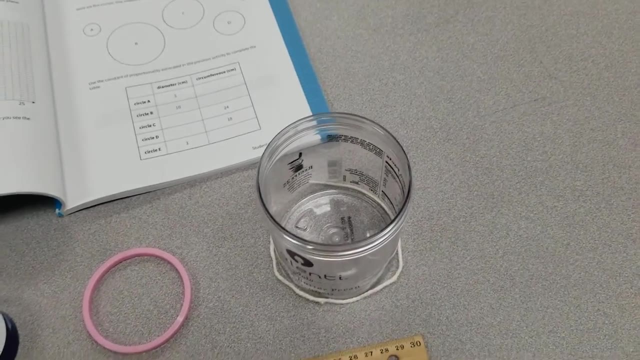 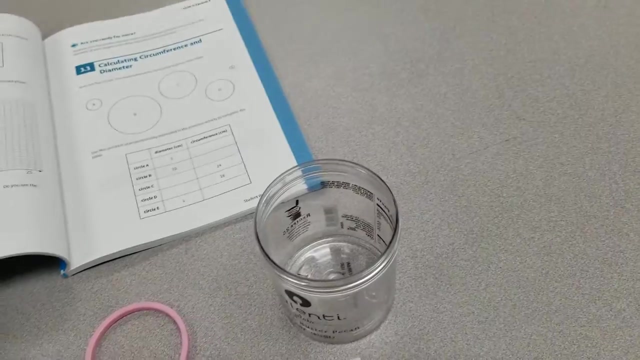 the way around my object. You can probably pick it up and use the string as a measuring tool. I've already pre-cut this string and I found that this string goes all the way around my object here. After that, I want to use my centimeters to measure the length of. 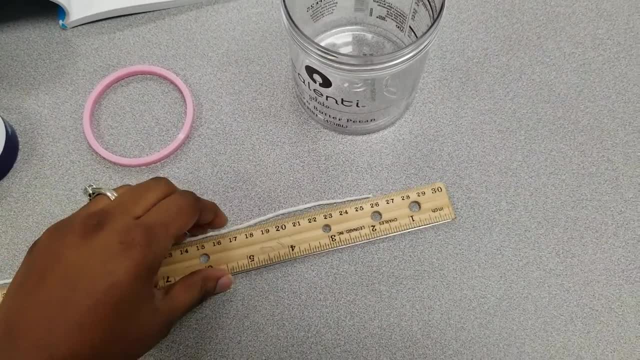 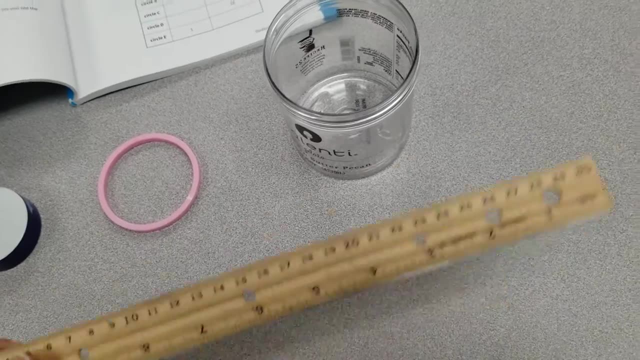 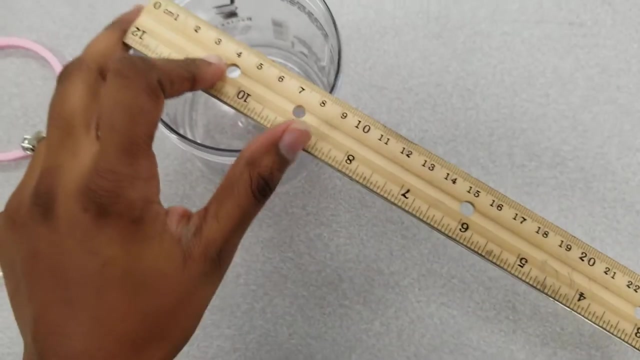 the string and the length of the string should be the circumference of my object. Once I've done that, I'll also take my ruler and measure the diameter of my object. So even though this is a cylinder, it does have- because this is a cylinder- it has a circular base. So 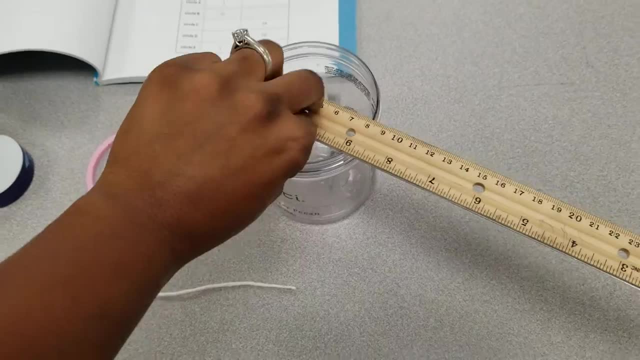 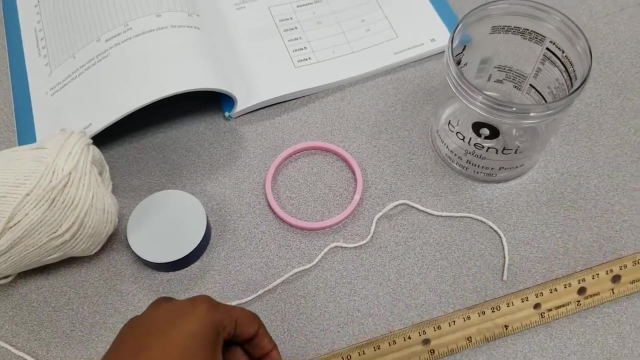 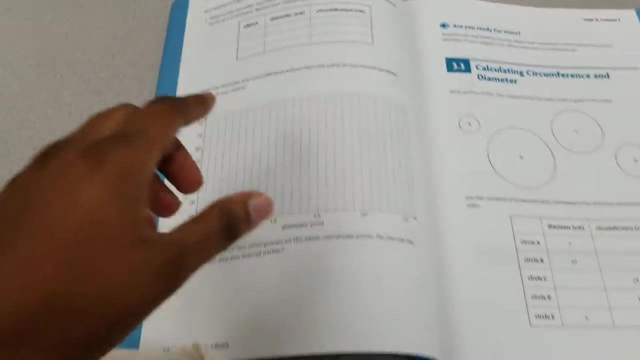 I can use this also to measure as a circle. Once I have my circumference and my diameter of my object, I'm going to write it into the page of my book And I'll follow the same process for all three objects, And then I'll.